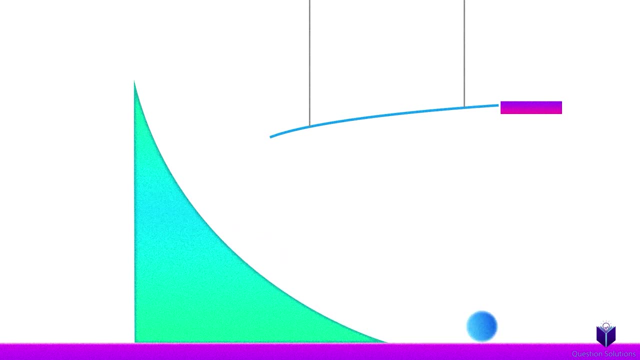 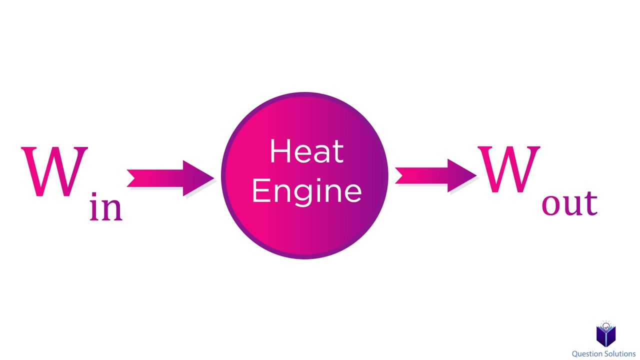 some work on it. The system can come back to its original state if it's irreversibly idealized. By thinking about idealized, reversible processes, we can figure out theoretical maximums for different systems. Remember that for a heat engine cycle the net work can be maximized by processes. 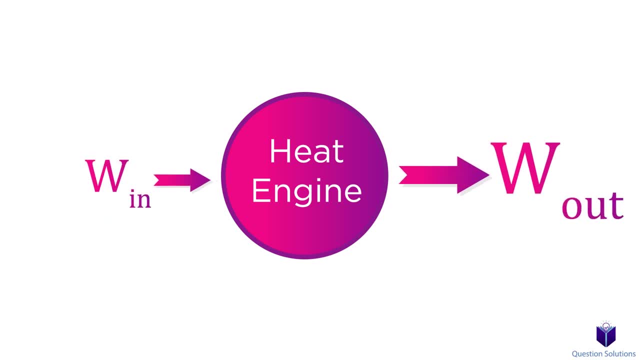 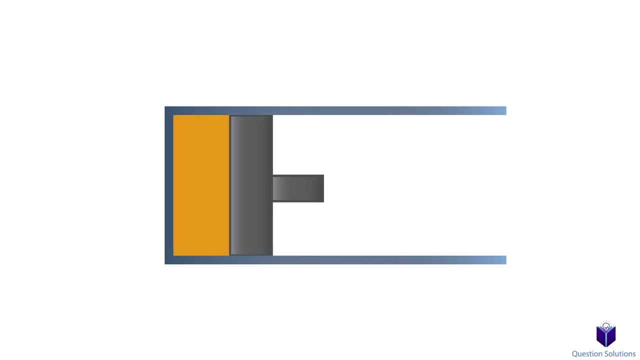 that require the least amount of work and deliver the most. This can be done by using a reversible process. In fact, the most efficient cycles are always reversible cycles. The most efficient cycles are always reversible cycles. The most efficient cycles are always reversible cycles. 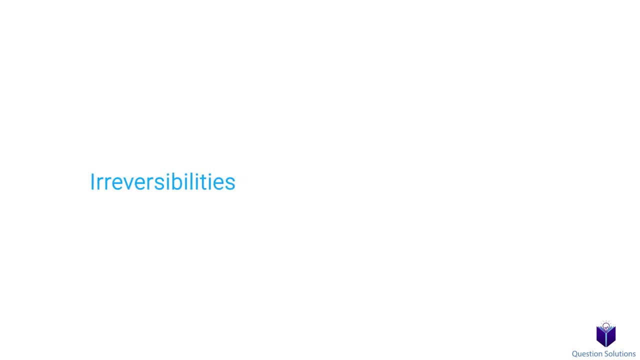 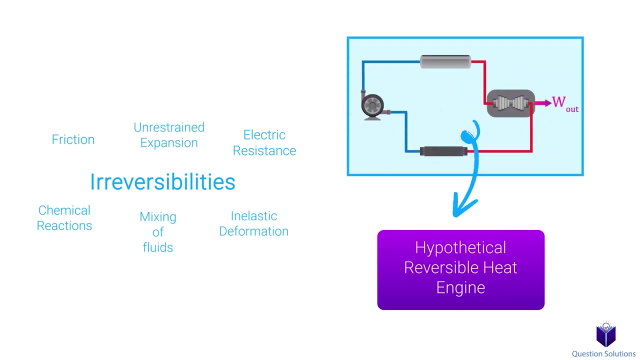 Now we know we can't actually achieve a reversible cycle in practice due to irreversibilities, But we can compare our existing heat engine to this hypothetical reversible heat engine. One such reversible cycle is called the Carnot cycle, proposed by a French engineer named Sade de Carnot, A heat engine that can be used to work on the 궁 parle. 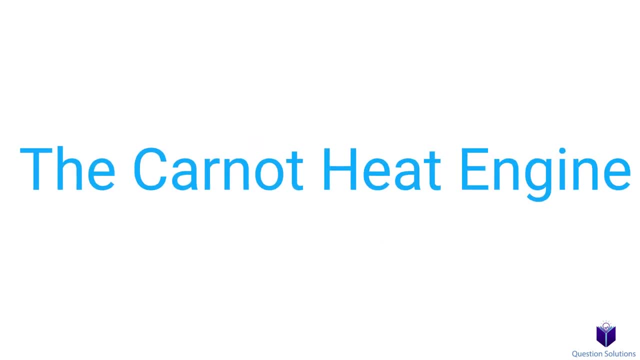 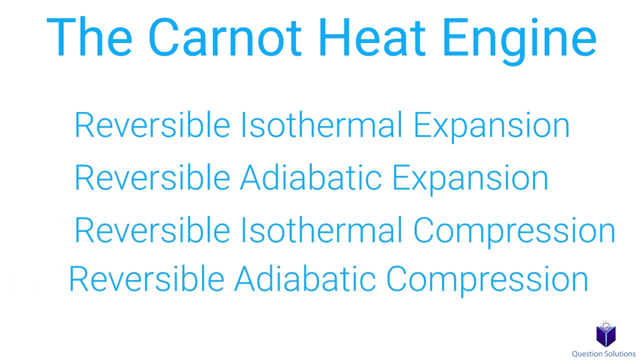 carnot signal is called a Carnot heat engine. A heat engine that operates on the carnot cycle is called a carnot heat engine. It has four reversible processes and it can work in closed or steady secondaryheheَ angles. It can be used to calculate heat per second. It's done by a logistic 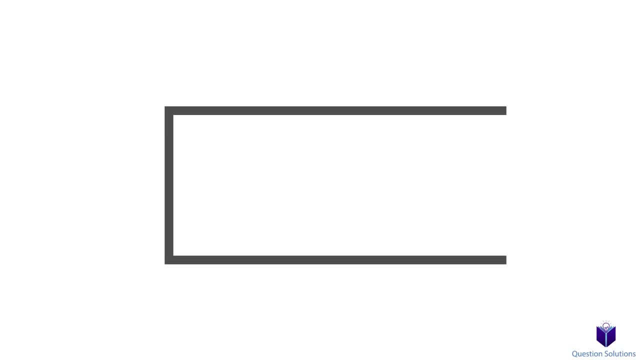 scale. All of these are ins: SolidW managingFLint. Now we know we can't actually achieve a reversible cycle in systems. Let's go through this cycle. Imagine we have a closed system with a gas inside a piston cylinder device. The first step of the cycle is the reversible isothermal expansion. Let's label: 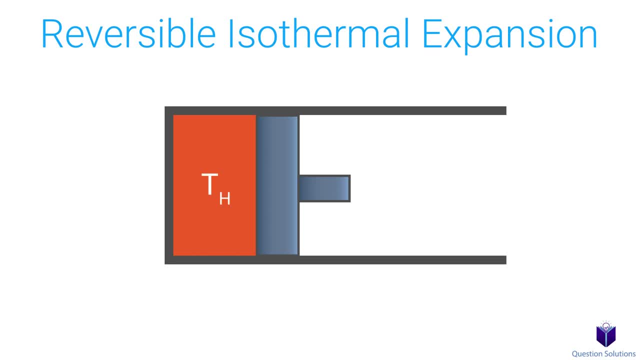 the temperature of the gas TH. The cylinder head, which is this part right here, is close in contact with an energy source. This source also has a temperature of TH. So, in simple terms, the temperature of the gas and the energy source temperature is the same. Now the gas inside is. 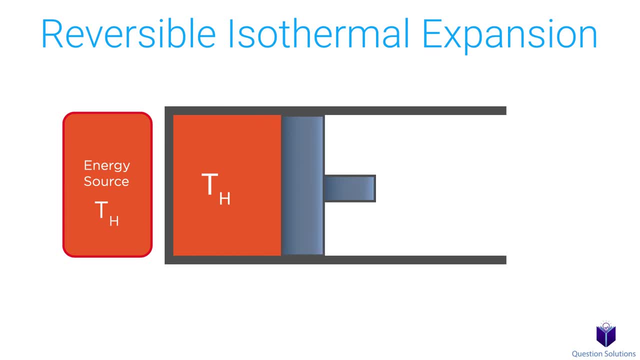 allowed to expand. When the gas expands, it does work on the surroundings. So here the piston moves to the right. As the gas is expanding, the temperature of the gas begins to decrease, But heat is transferred from our energy source back into the gas. This means the gas temperature stays. 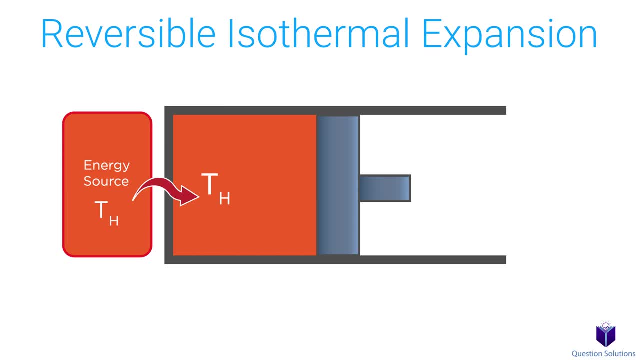 constant at TH, Because the temperature difference between our energy source and the gas never changes more than an infinitesimal amount. this is a reversible heat transfer process. The total amount of heat transferred during this step we can label QH. The second step is called the reversible adiabatic expansion. At this step, 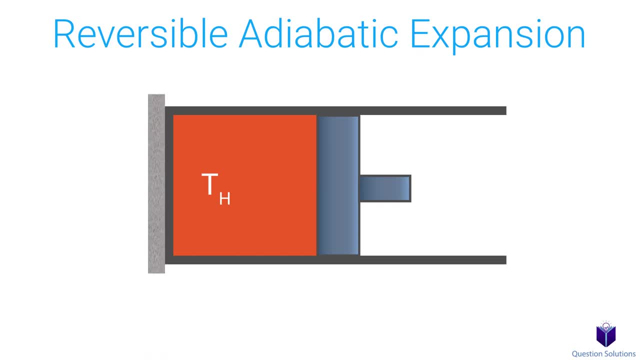 we remove the energy source and replace it with insulation. The system then becomes adiabatic. Adiabatic just means there is no heat transfer to or from the system, So the gas in the 불� 퍼 is full. It's like a tienes Veronica Electric. 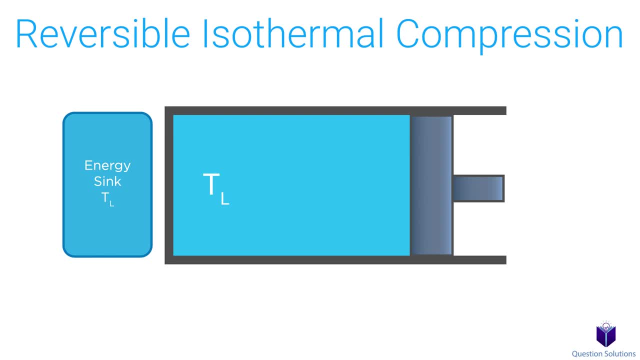 At this point, when we get in contact with an energy sink, we have no energy source, but we can. we can connect thefunction. We're using a face circuit. We use the đấyes metric to provide absolute capturing of energy loss. As a result, the gas remains constant throughout the 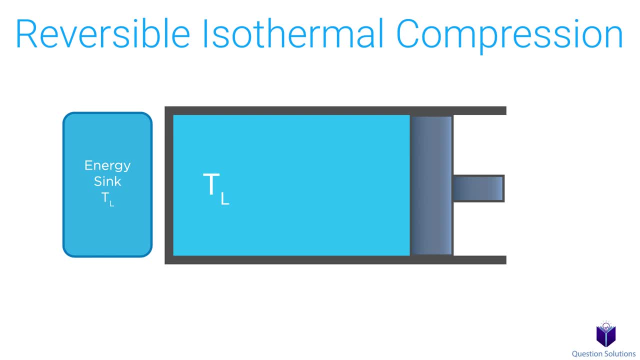 system. The gas still expands and drops in temperature. We will label the new temperature we place is at the same temperature as the gas. Now an external force pushes on the piston, moving it to the left. This causes the gas to compress and the temperature begins to rise. 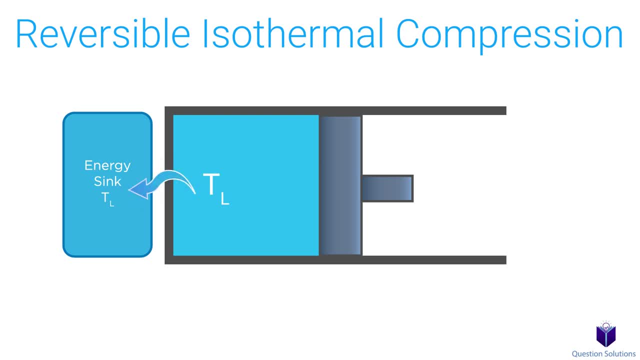 But as soon as it's rising, the heat is transferred to the energy sink. So the temperature of the gas remains constant at TL, Because the temperature difference between our energy sink and the gas never changes more than an infinitesimal amount. this is a reversible heat transfer process. 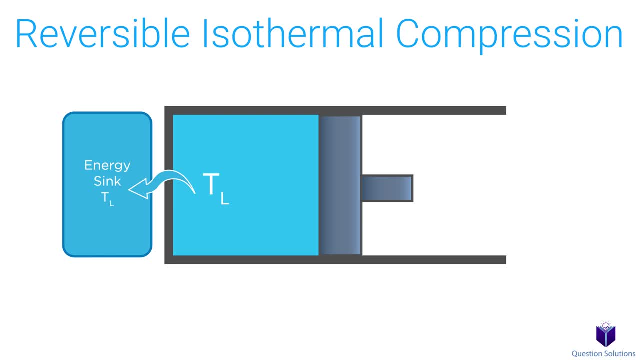 The total amount of heat rejected from the gas during this step we can label QL. The fourth and last step is called the reversible adiabatic compression. Now the low energy sink is removed and insulation is placed back on the cylinder head. 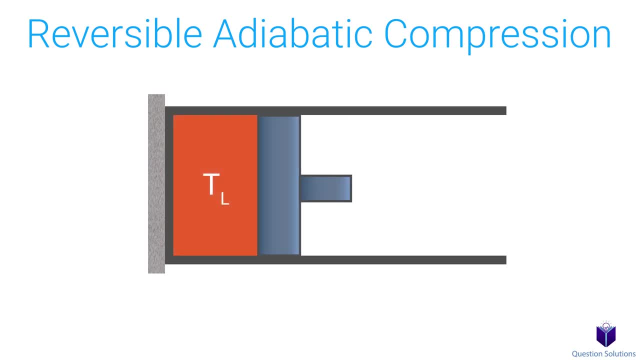 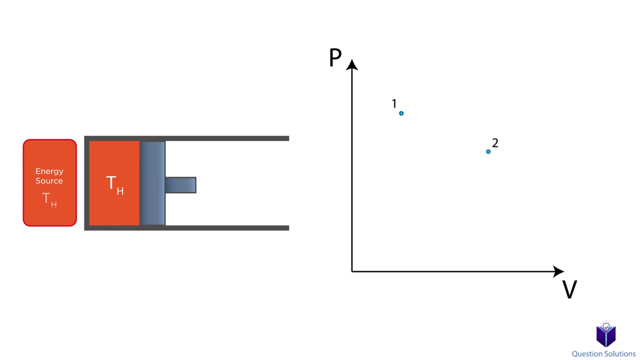 The gas continues to be compressed and it goes back to its initial state. In other words, the temperature rises from TL to TH, which means the cycle is now complete. Let's look at a pressure-volume diagram of a Carnot cycle Starting from step 1 to 2,. the pressure drops and the volume increases as the 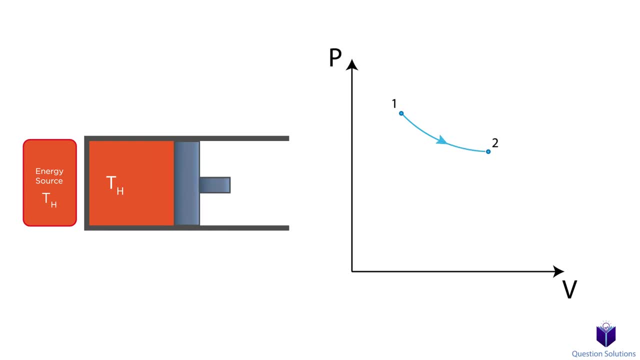 gas expands, The temperature stays constant at TH. For the temperature to stay constant, heat needs to be transferred. so we have QH, which is the heat transferred from our energy source From step 2 to 3, the pressure drops more and the volume increases as the gas expands. For the temperature to stay constant, heat needs to be. 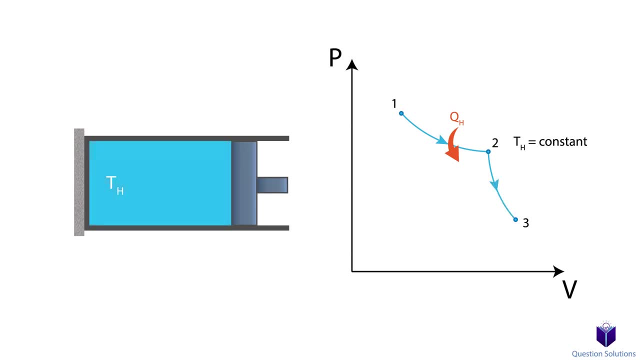 volume continues to increase Because our cylinder is now insulated. the temperature drops to TL From step 3 to 4, the piston is pushed inwards, so the gas is compressed, The pressure increases and volume decreases. There is an energy sink, so the temperature is kept constant at TL. 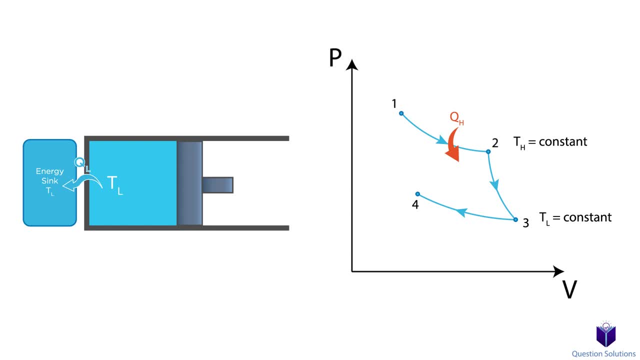 For that to happen, heat needs to be rejected into the energy sink. so that's QL From step 4 to step 1, we insulate the cylinder while the piston keeps pushing inwards, The pressure continues to increase and volume continues to decrease. 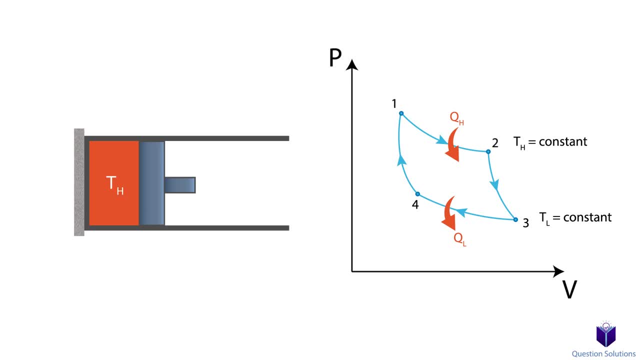 arriving at the same state as step 1 and the temperature rises to TH. The area inside the path 1-2-3-4-1 shows us the network done during the cycle. Keep in mind that the Carnot heat engine cycle is a reversible cycle. 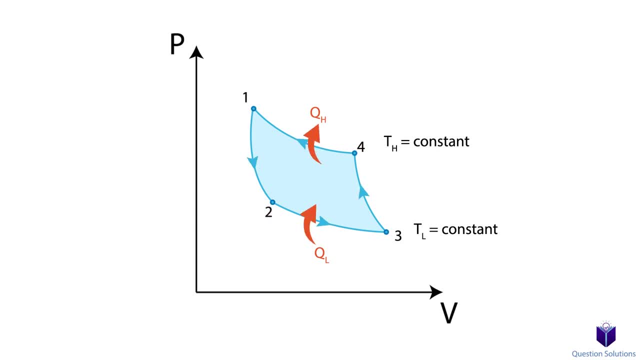 so every step can be reversed, Which would result in the Carnot refrigeration cycle. Here is the pressure-volume diagram for a reversed Carnot cycle. The biggest difference lies in the direction, along with QL being the heat absorbed from a low-temperature reservoir and QH being the heat rejected to a high-temperature reservoir. 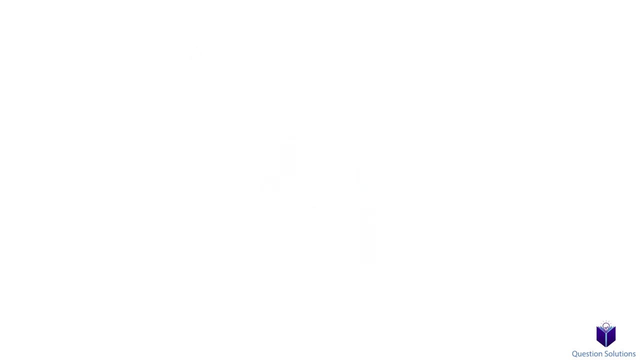 Now let's dive into the efficiency of a Carnot engine. In the previous heat engines video we talked about this equation, which gives us the efficiency of any heat engine. Here, QH is the heat transferred to the engine from a high-temperature reservoir and QL is the 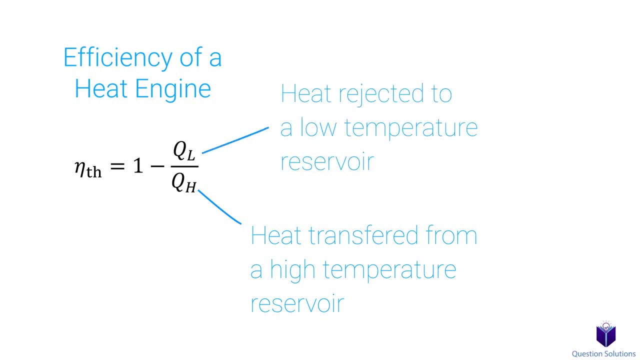 heat rejected to a low-temperature reservoir. When it comes to reversible heat engines, like the Carnot engine, we can go one step further and write our efficiency equation like this: Remember that TH is the temperature of the high-temperature energy source and TL is the temperature of the energy sink. 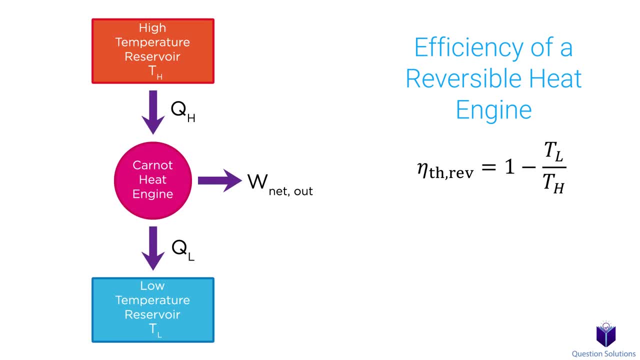 This relation is called the Carnot equation, the Carnot efficiency. In simple terms, this equation says the efficiency of reversible engines is a function of reservoir temperature only. You should note that TL and TH must be in Kelvin for this equation to work, because they are absolute temperatures. Do not use 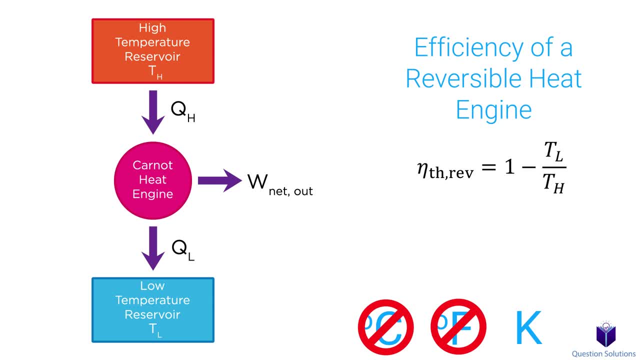 Celsius or Fahrenheit when solving problems, or you will end up with incorrect answers. A relationship between our Carnot efficiency equation and the normal efficiency equation can be written like this for reversible heat engines: Again, the values must be in Kelvin for this equation to work. 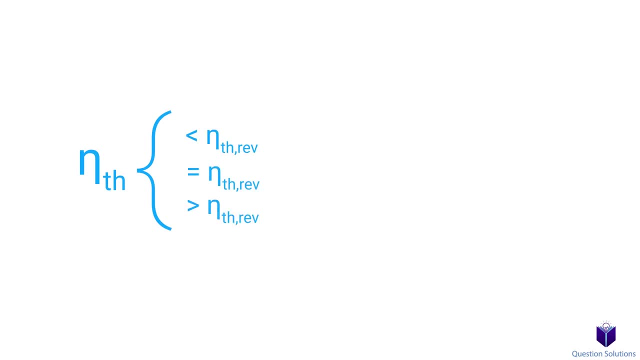 If we compare the thermal efficiency equation to the Carnot efficiency equation, we can determine what type of heat engine it is. If the thermal efficiency is less than the Carnot efficiency, then it's an irreversible heat engine. If it's equal to the Carnot efficiency, 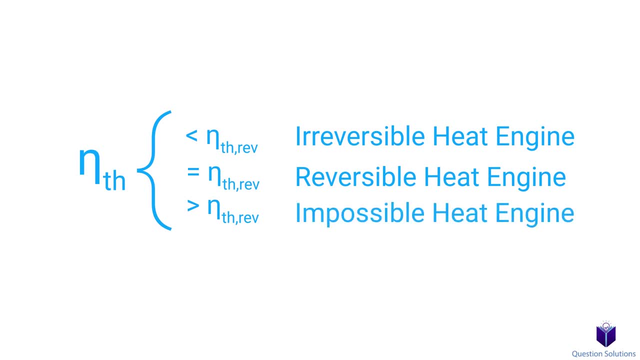 then it's a reversible heat engine, and if it's greater, then it's an impossible heat engine. Subtitles by the Amaraorg community. Now let's go through some problems to see how we can apply what we learned. Let's take a look at this question where we have a Carnot heat engine that receives 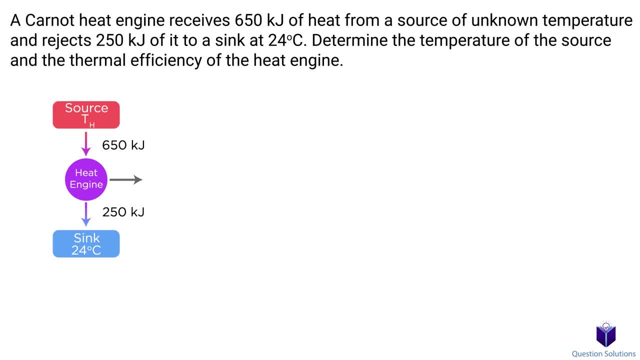 heat from a source where we don't know the temperature. We need to figure out the temperature of the source and the thermal efficiency of the heat engine. Let's start by writing down what we know. The engine receives 650 kJ of energy and rejects 250 kJ, So that's our QH. 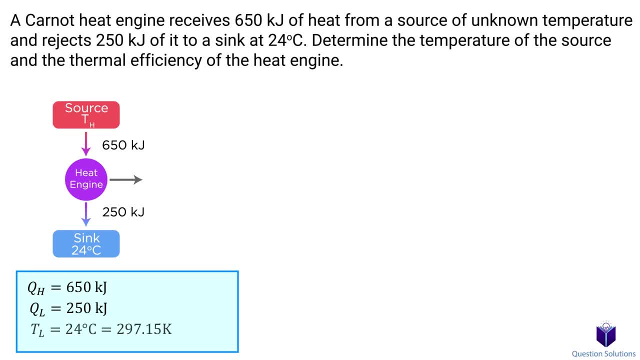 and QL. The sink where heat is rejected to is at a temperature of 24 degrees Celsius. We can use this equation to figure out the temperature of the energy source. since this is a Carnot engine, Let's plug in the values we know. Solving gives us the temperature of the energy. 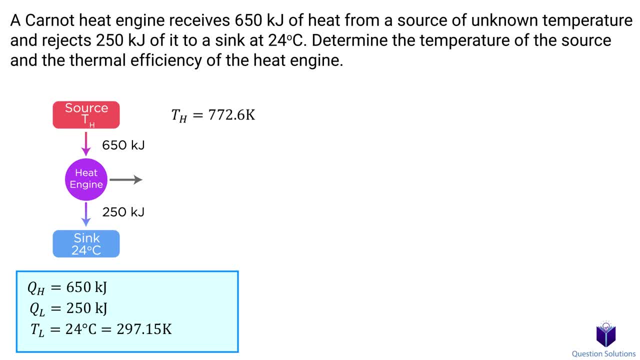 source. We can find the efficiency using the Carnot efficiency equation. So let's plug our values in, and those are our answers. Subtitles by the Amaraorg community. Subtitles by the Amaraorg community. Subtitles by the Amaraorg community. 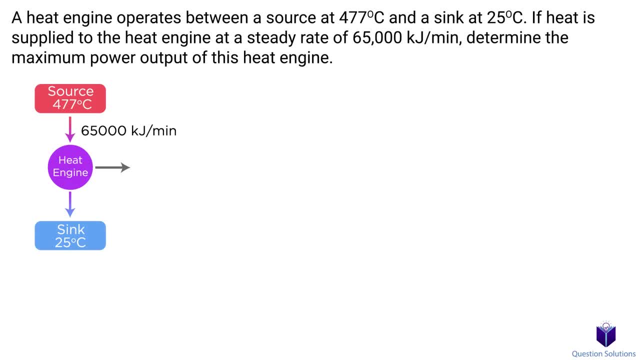 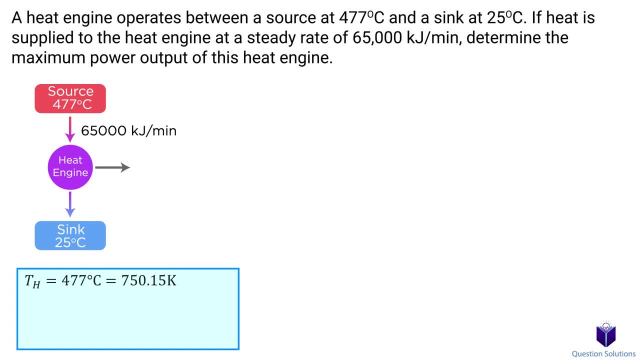 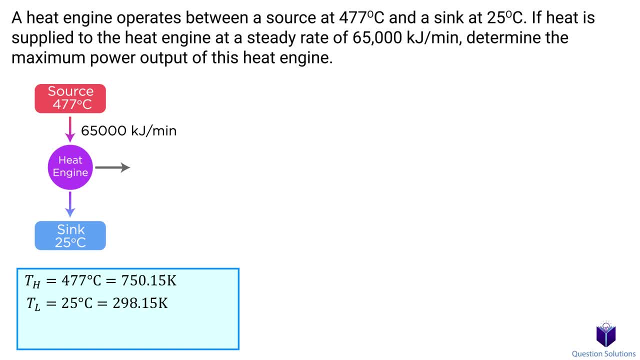 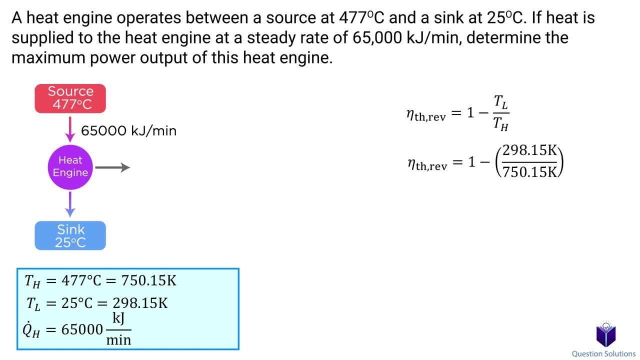 the Carnot efficiency equation. Let's plug our values in and that gives us our efficiency To figure out the maximum power output. we need to use this equation. You should remember this from the heat engines video. Here our Q in is the heat supplied. Let's rearrange. 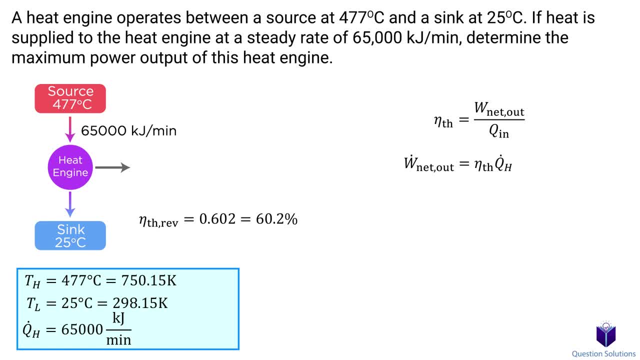 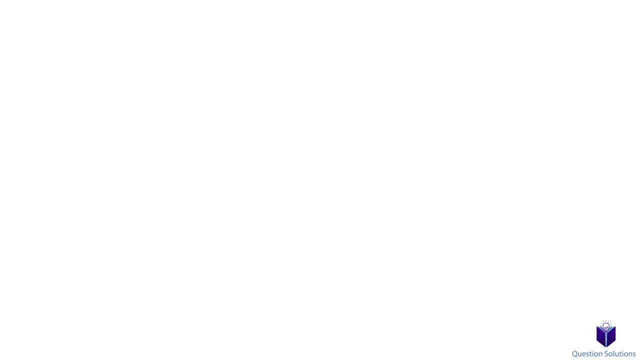 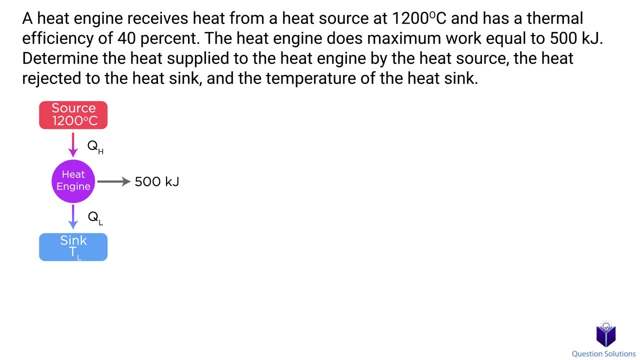 the equation and write it in time rate form. Now we can plug our values in and solving tells us the maximum power output. Let's take a look at this problem where we have a heat engine that does maximum work equal to 500 kilojoules. We need to figure out the